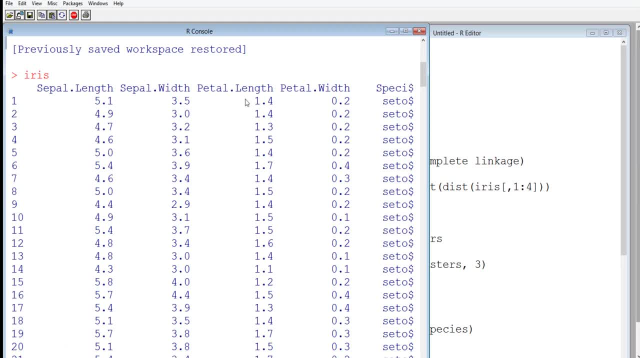 All right, So we've got sepal length, sepal width, petal length and petal width, and species Species is the level, But we'll consider as if this data is unlevel and we'll just, you know, remove this variable while building the model. 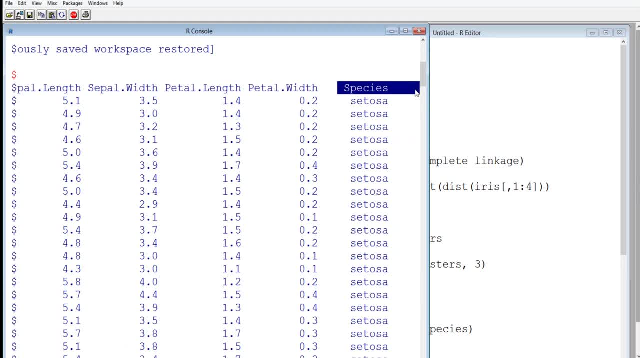 And later on we'll just compare it with the actual data. So, using the length and width of the flowers, we'll try to find out the correct clustering or how many clusters of flowers we have. You know, the idea is to find out clusters in the datasets. 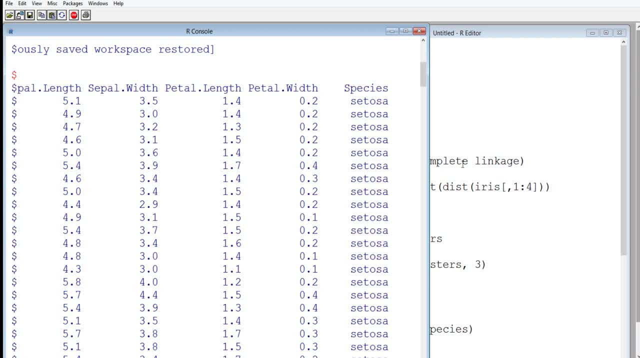 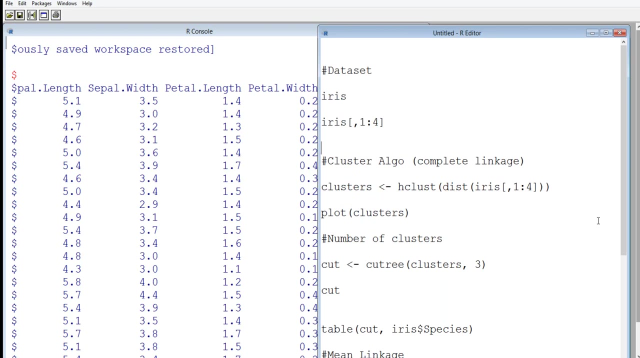 Right. So we'll expect three clusters, because we know beforehand. But you know, in most real-life scenarios you won't know how many clusters are present, So that's slightly more difficult to find out. So one of the big difference, or the main difference between k-means and the hierarchical clustering is that in k-means we need to know the value of k. 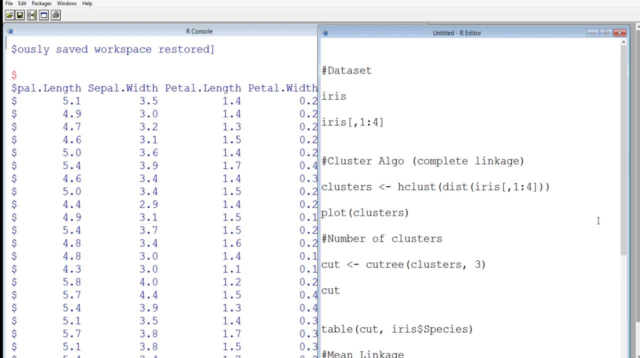 That means the number of clusters present- or we at least think about the data to be present in the data. So we need to know how many clusters could be there in the data. OK, so that's one big difference here. in hierarchical clustering, We need not provide the algorithm as to how many clusters we think the data would be having. 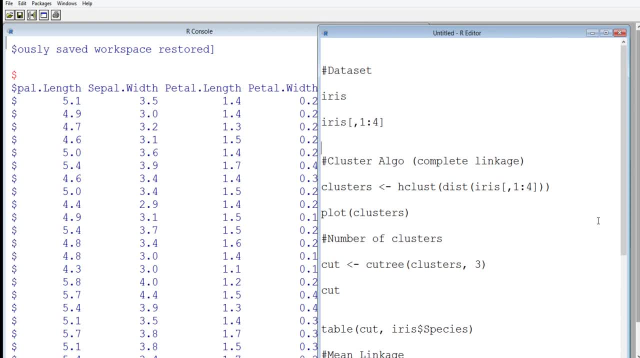 So that's something that we find it out by running the algorithm, So we don't need to know about it. So that is more exploratory in nature. This is more exploratory. That means we explore the number of clusters. We also explore which observation belongs to which cluster. 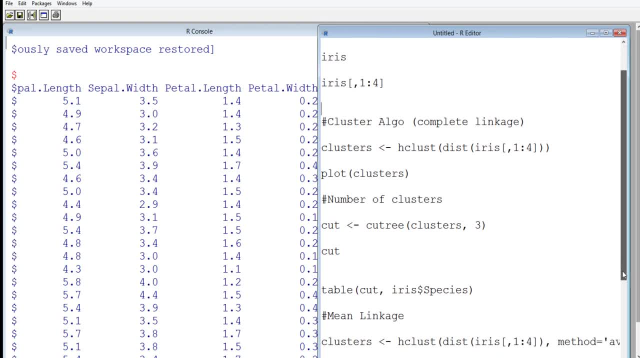 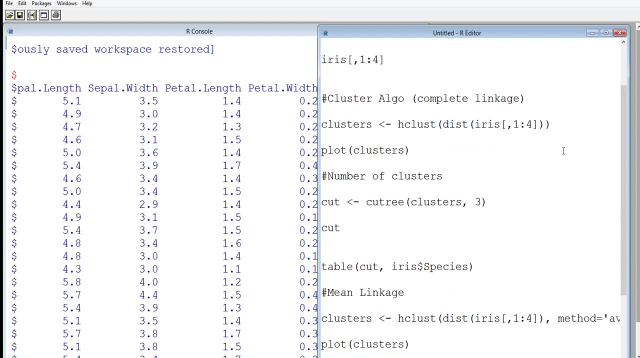 OK, so that's one main difference. The second important thing I'll talk about here is that The way we calculate distance between two clusters. So in the theory section there is a video in this description section where I've explained how we calculate the distance between different clusters. 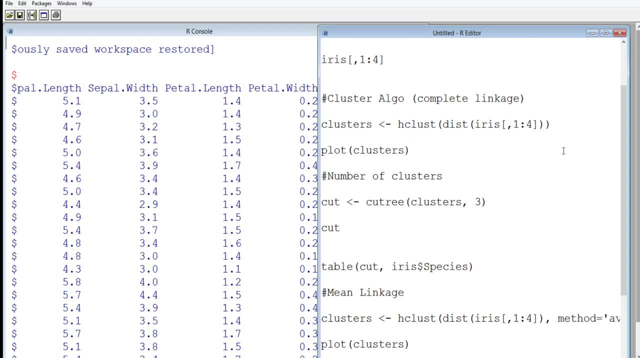 There are many ways. Two important ways is to take the extreme points to farthest point, And then the other way could be to take the two nearest points and take the distance, And the third way could be to take the average distance. So, by default, the function that we are going to use, hclust, which will do the hierarchical clustering. 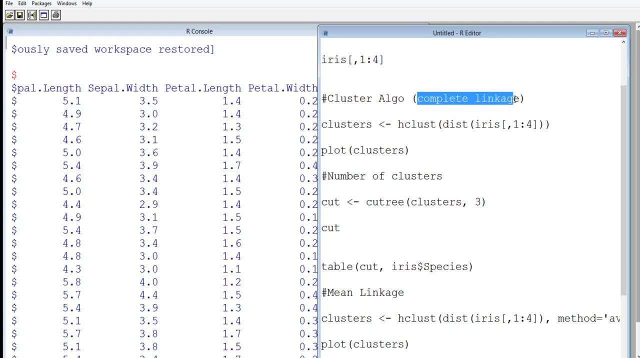 By default it does complete linkage. That means the way it calculates the distance between clusters is just by taking the distance between the most extreme points or the farthest points. OK, so that's by default. We don't have to explicitly specify this. 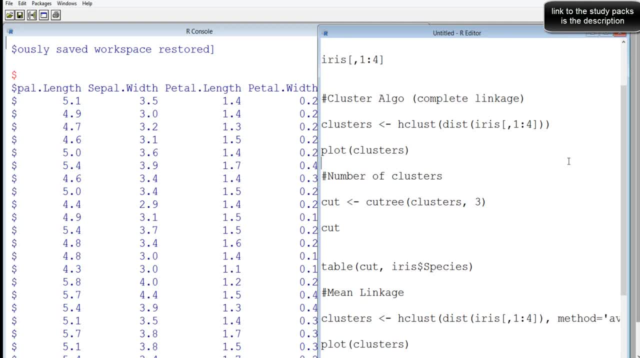 We'll see. you know some other ways also, just for comparison as to which one does a better job. So the function that we will use is hclust And we're going to have the iris data, And we will take only the first four variables right. 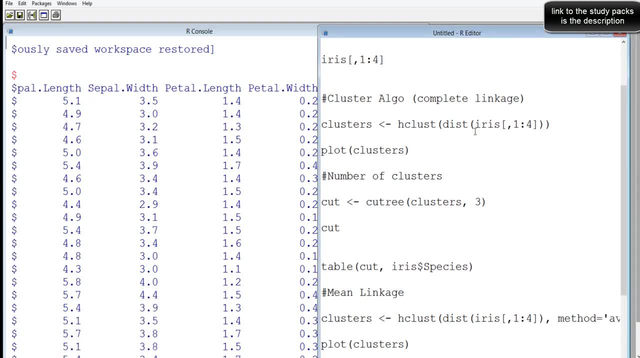 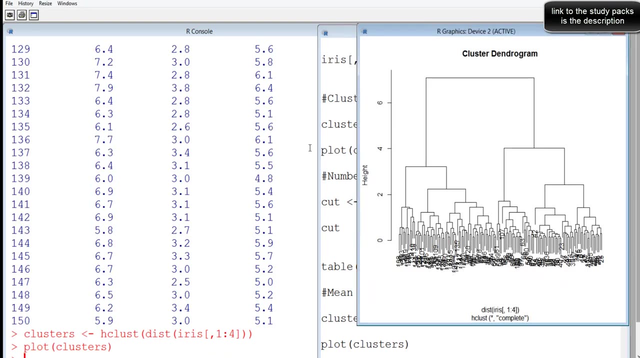 Sepal length, sepal width. petal length, petal width. That's why we have done this subset of it. OK. so let's run this. In the second step, we will try to plot and we will see how many we can consider to be having. you know, clusters. 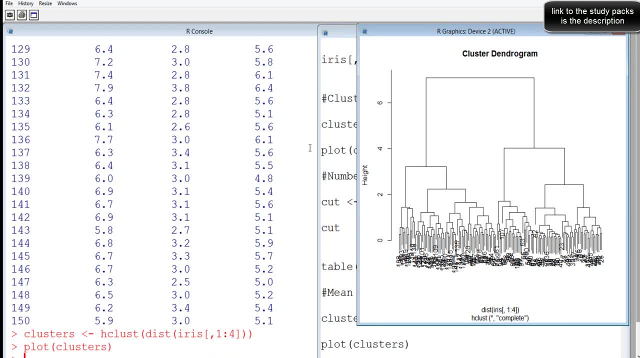 So how many clusters do we do? we think that is present in the data, So I've got you know clearly. Clearly there are, you know, two clusters, very clear. So this one you can see, the left one and the right one. 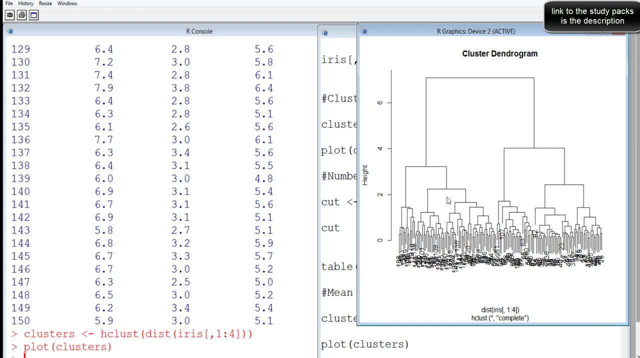 Out of the below two ones, if you see the bigger segments, one of them could be a cluster, OK, but we are not very sure. Two is very clear, Or three also could be one of the case. So we will see two and three. 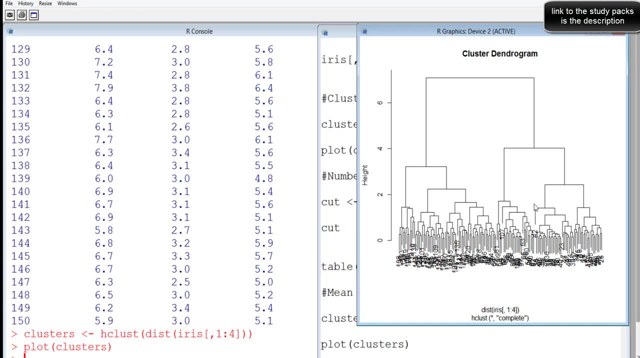 So beforehand we know that there are three clusters because there are three species of data. So we can go ahead. We can go ahead with, you know, subsetting it for three. But in more exploratory analysis, where you know you do not know for sure how many clusters are there, 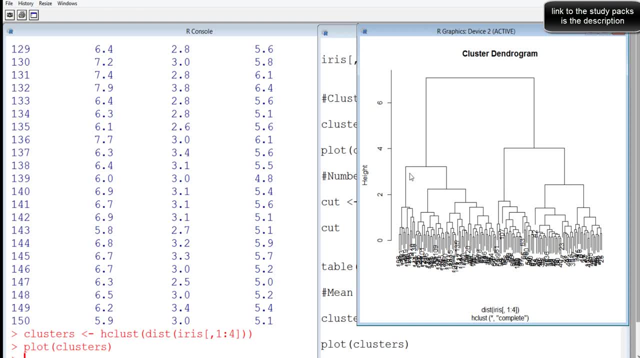 what you do is that look at the way that you know the segmentation has happened And you only take the ones. that is, you know clearly visible to be different. So here you can see a smaller one, So you can take the complete one. 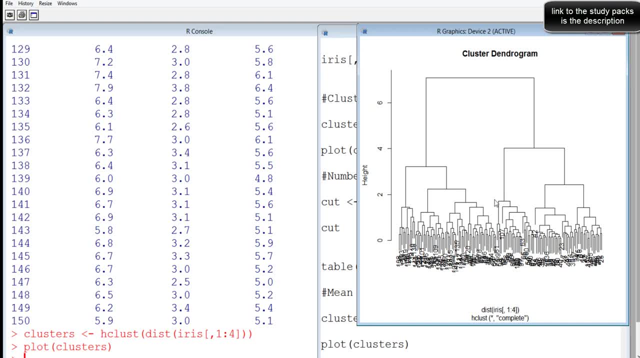 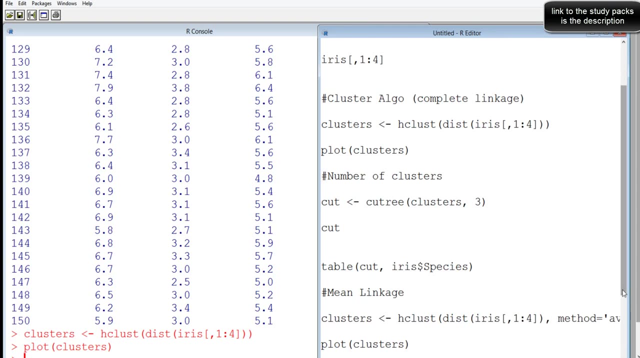 Here it is slightly bigger And you can take this one as one cluster and the other one as another cluster. So there could be three clusters clearly. So just by looking at, you know, this dendrogram, we are sure that one of the clusters that we expect to be clearly, you know, visible in the data is not very visible. 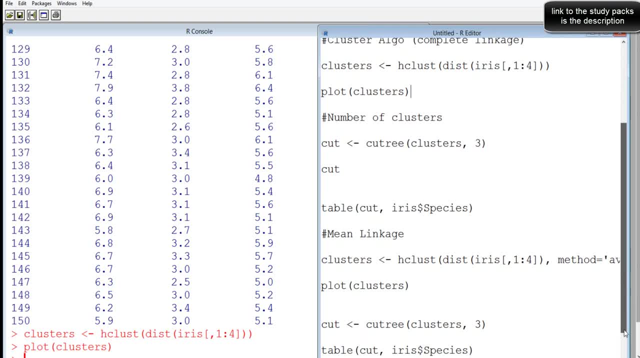 And we will see that just by doing a cross-validation. So we will take three clusters out of it, The way we take three clusters out of several clusters that we just saw. Okay, so let me show you the plot again and a few more things to note here. right? 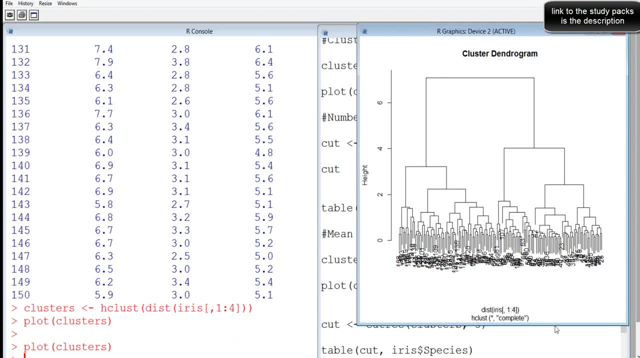 So in hierarchy cluster, we will have many number of- you know, clusters and sub-clusters and so on, Till the point that each observation is a cluster. So in total we have 150 clusters. to be precise, If you have 1000 observations, you will have 1000 clusters. 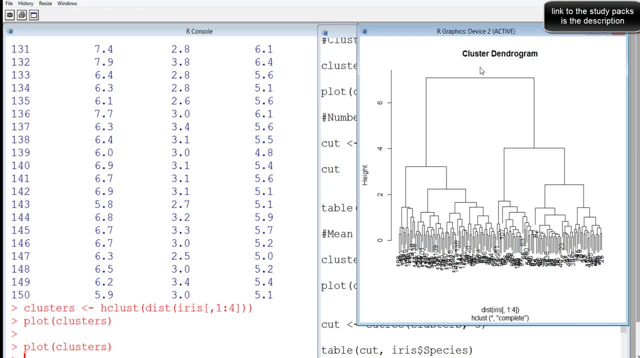 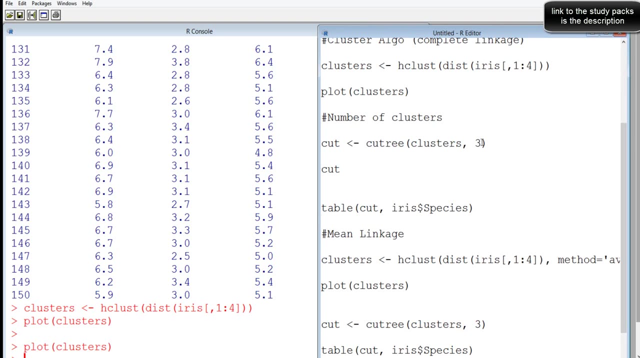 But important thing is to you know: choose from top, Okay, The bigger one will get the higher precedence while selecting the number of clusters. So you have flexibility. Okay. So we will go with three, Okay. So the second step is to do is to cut the tree. 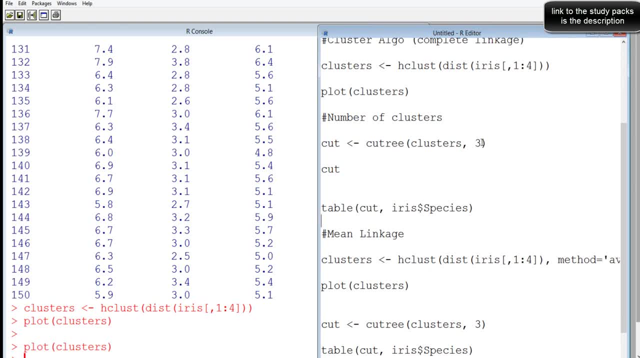 Just to have optimal number of clusters. We cannot have 150 clusters for 150 observations. We will cut it down for three, So the function that we will use is cutTree. Okay, So we now cut it down to only three clusters. 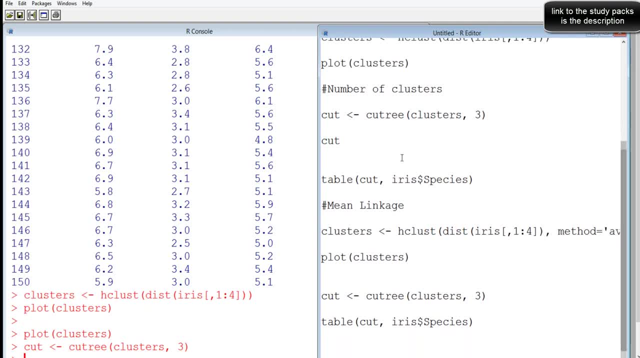 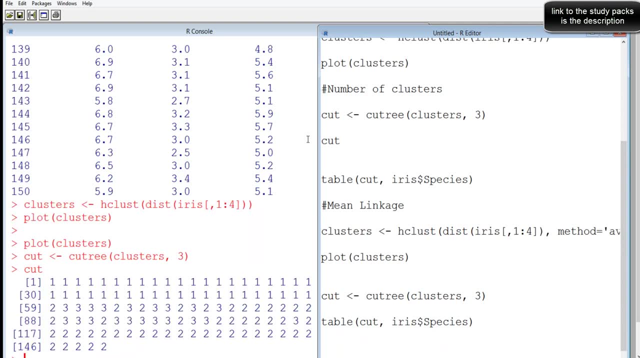 Because that's the optimal we believe, Okay, Okay, So what's there in the variable? So, whatever? So the entire 150 observations are now being clustered into three groups. Okay, So if you just make it like let's say four, you will see it will be four groups. 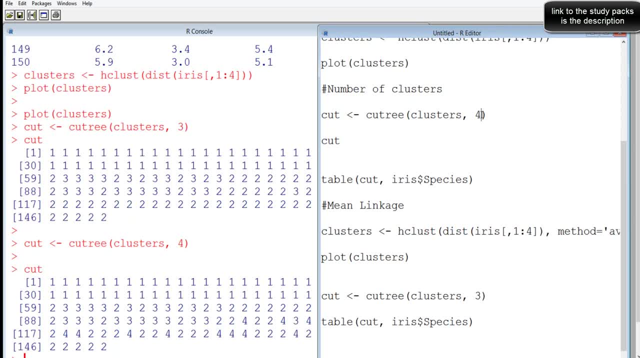 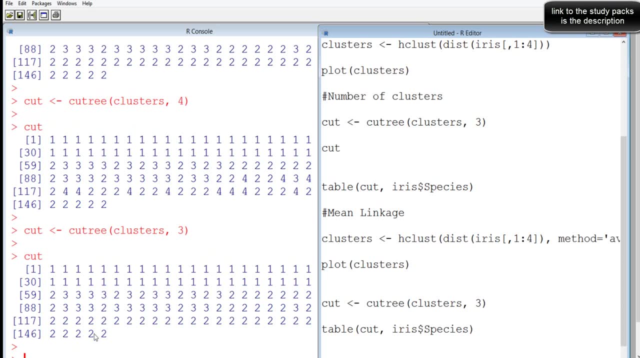 Now you have one, two, three, four, Right. So if you just keep it to three, Then we'll have, you know, only three clusters: One, two and three. All right, So the next thing to do is to do some sort of a cross-validation. 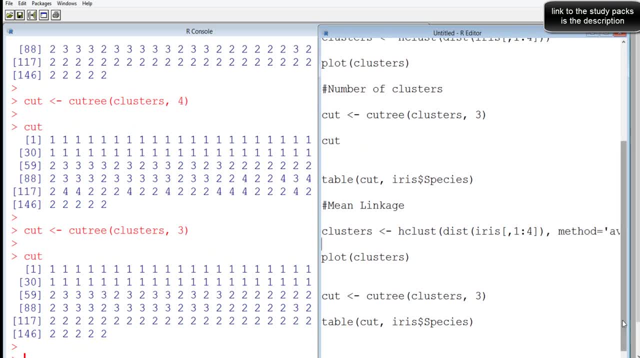 Now, that's the luxury we have here, because the data here is level. But in many situations you won't have that luxury. You won't have a level data to you know. do cross-validation Sometimes you have. you may not have a complete or a large set of level data, but you may. 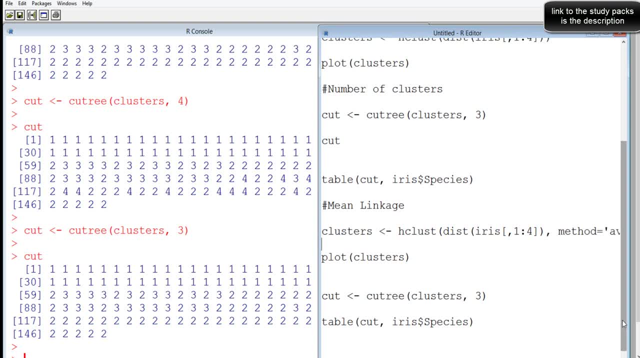 have a small set of level data. Even there you can do the cross-validation. That's also a good way of knowing whether clustering is perfect or not. So we will do a cross-validation by taking the predicted cluster and the actual cluster. The predicted clusters is there in the variable cut. 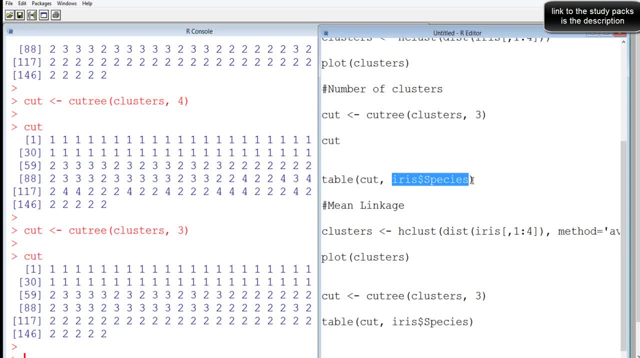 The actual clusters are present in the iris species, Right? So it's iris data. We have this variable species which has got the three different types of species. So you do a tabulation. You do a tabulation of that and see what's the result. 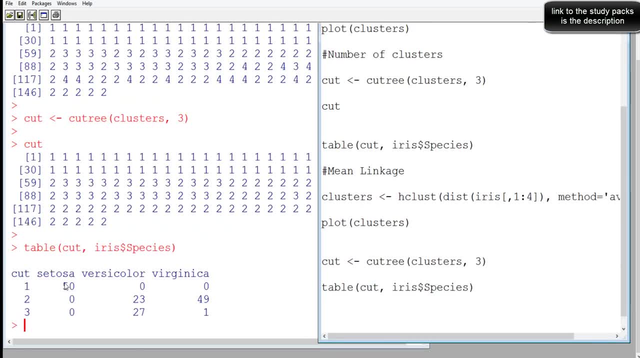 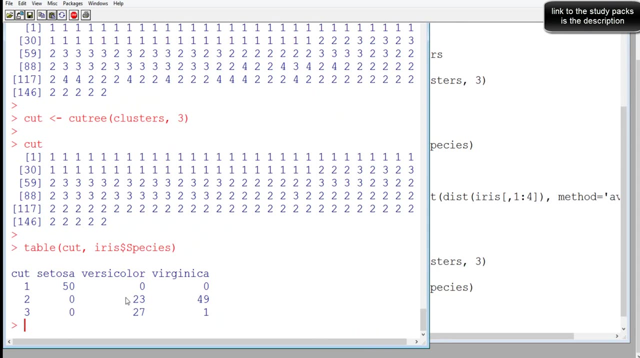 Well, you can see that all cytoses- 50 out of 50, have been correctly classified. The virginica- 49 of them- have been correctly classified. One out of them is not very correctly classified. Versicolor is the one which is getting affected the maximum. 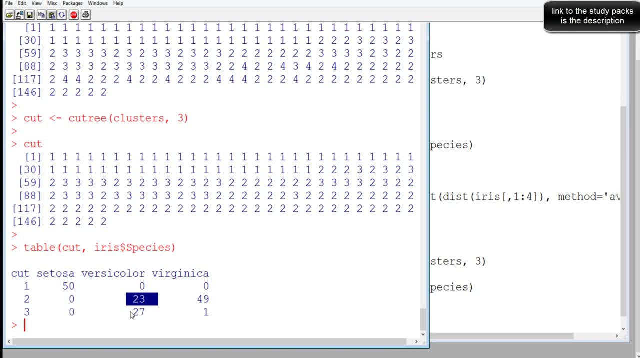 That means you know there is a large classification error. You know which is close to 50% classification error. that's happening in verticolor. Only 27 have been correctly classified, 23 have been incorrectly classified. So that's a clear issue. 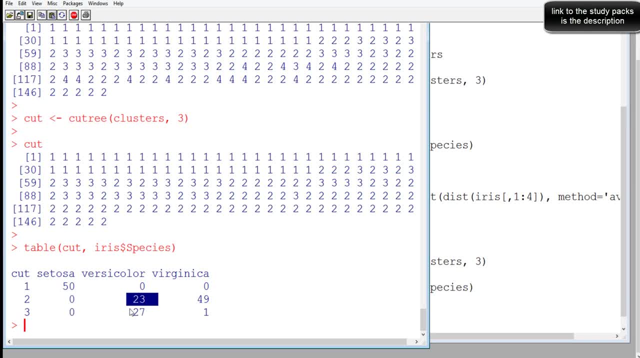 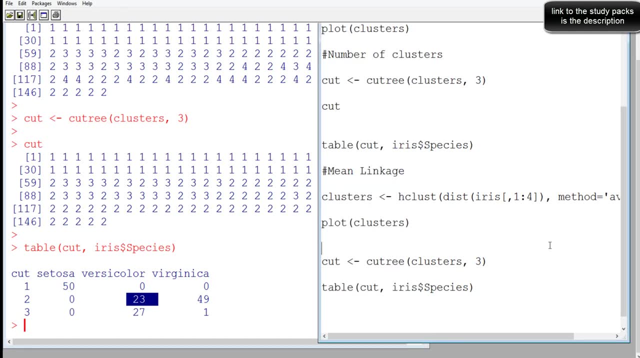 As we are expecting. one of the you know cluster that we were expecting to be very clear is not very clear. Even on the dendrogram we saw that's not clear. So we can try other linkage methods, Like the way distance is being calculated. 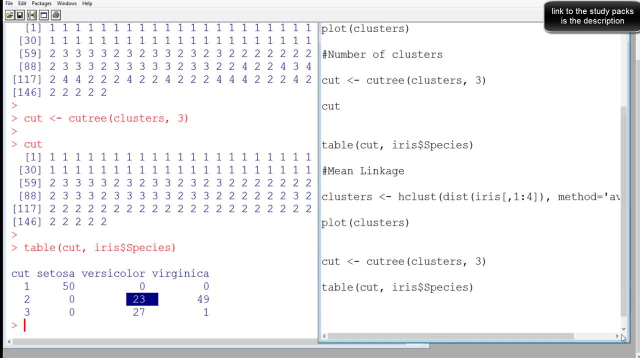 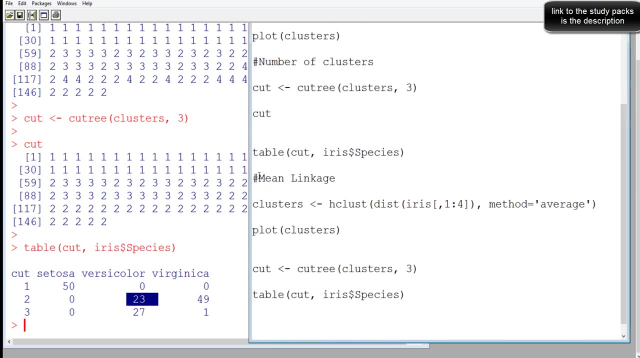 Between two consecutive clusters while doing the merging. Okay, So we will take the average linkage method. So we make very small change to the syntax. So the syntax remains same, except the fact that we have now used method equal to average. Okay, So in that case, 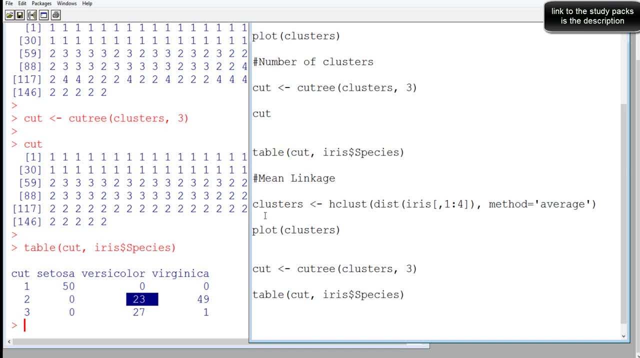 instead of a complete linkage which takes the distance between the two extreme data points in the clusters in the two clusters. while calculating the distance here, it will take the average distance of all data points with the corresponding data points in the other cluster. Okay, 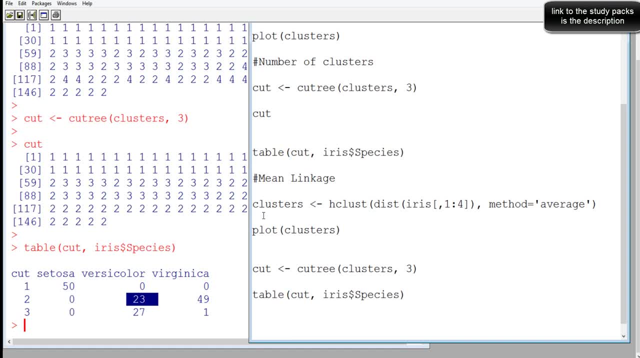 So for a better understanding of what these linkages are, I have a detailed explanation in the video, in the description. I will post that video on clustering. You will get a thorough overview of what clustering is all about and what the different linkages are, and so on. 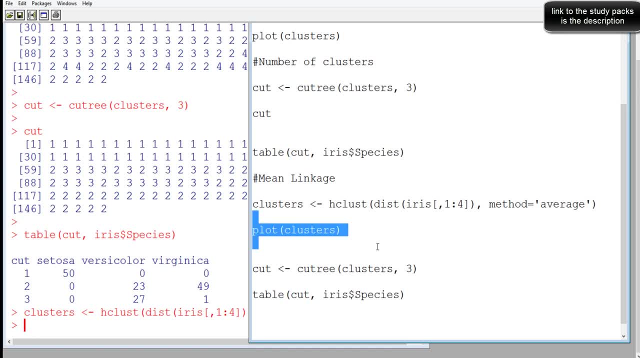 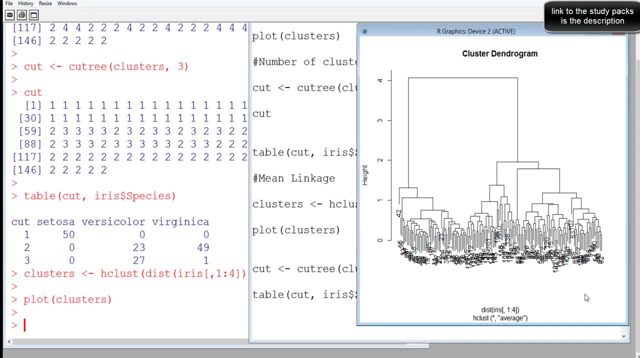 Okay, So let's run this. Okay, Then we will plot. So here we have slightly a better clarity Right. We can clearly see here that there are three clusters. One is here, This one, the leftmost one And the rightmost one. we have got two. 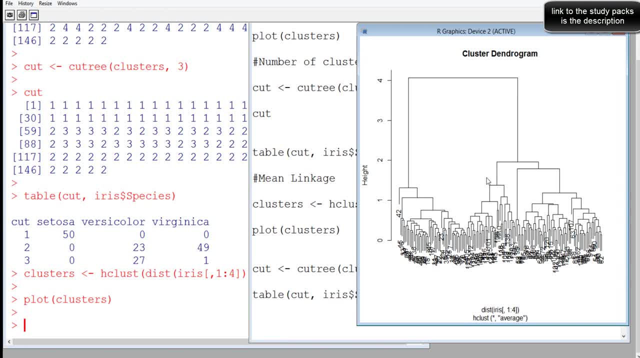 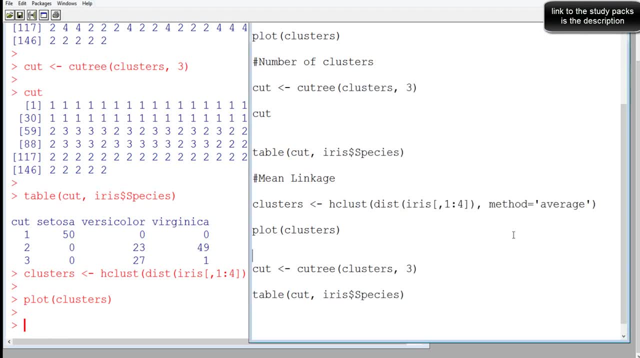 This one, If you can see my cursor, And the third one, This one Right, So we clearly have three clusters. This is a better diagram, So this seems to be working better than the complete linkage. So we will cut it down to three clusters. 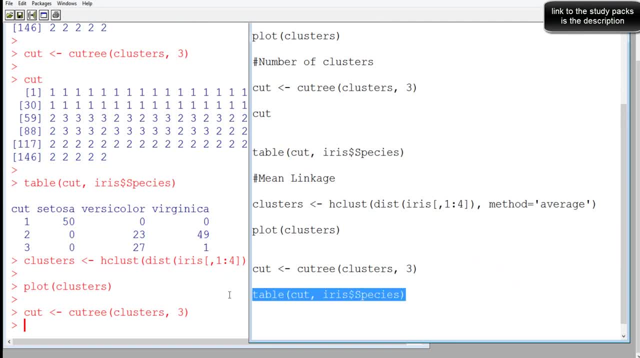 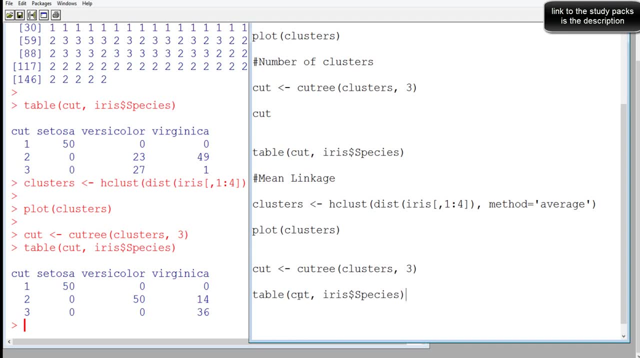 All right, And the next thing we will do is we will tabulate it. So we will tabulate the actual data with the predicted data. So the actual data is there. in iris species, the variable species, We have the predicted one in the variable cart. 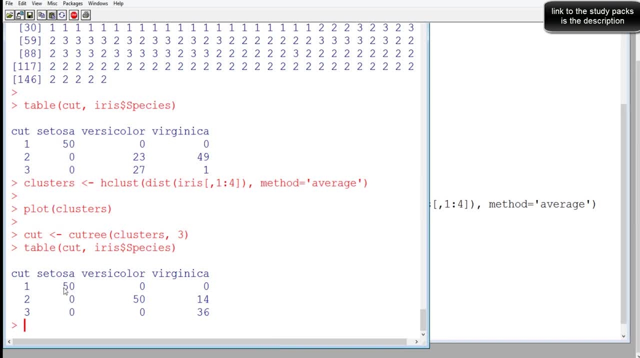 So now we see that all 50 sitosa have been correctly classified, 50 verticular have been correctly classified. Virginica is having an issue. Now we are facing a different issue, Right? So previously we used to have a correct classification of Virginica. 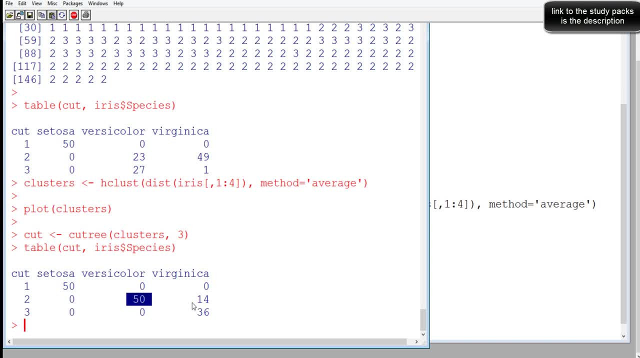 Mostly a correct classification. 49 out of 50 got correctly classified, But verticular had a problem. We had almost like 50% error rate, But here sitosa and verticular have been, you know, well classified. But Virginica is having an issue. 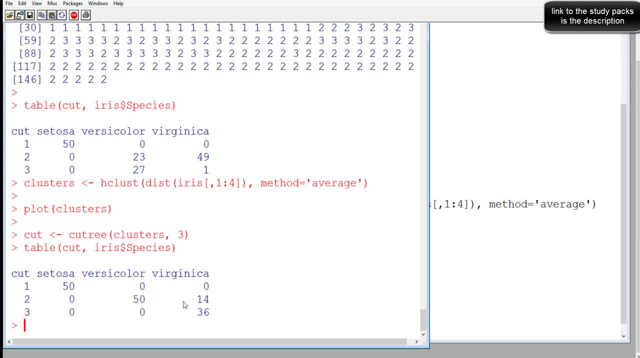 But the error rate is much less. It is, you know, somewhere around maybe 30%, 25%, 30%. So, depending on which category is more important from a classification point of view, we will choose which one to go with. Okay, 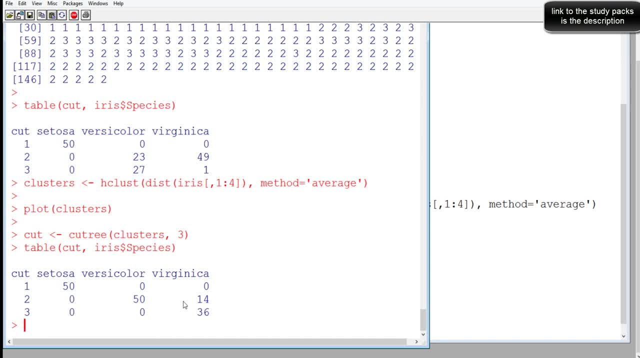 And there are many more methods also. We have only, you know, taken down the two ones. You can try out- you know other methods as well- And see which one is working fine. One other thing to keep in mind while building clustering model is that 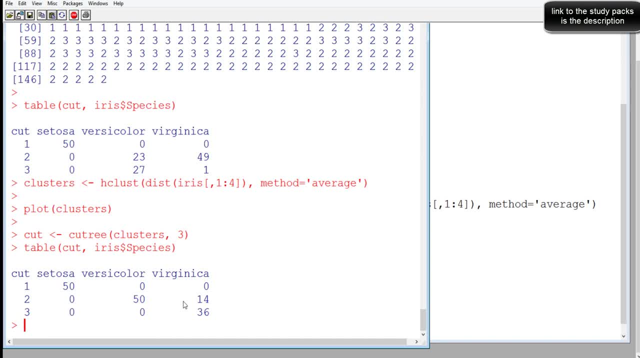 to try out as many clustering models that you possibly can try. You can also try k-beams clustering and see which one is working the best. Okay, Because cross-validation is a big issue in clustering. That's why it's always good to try out. 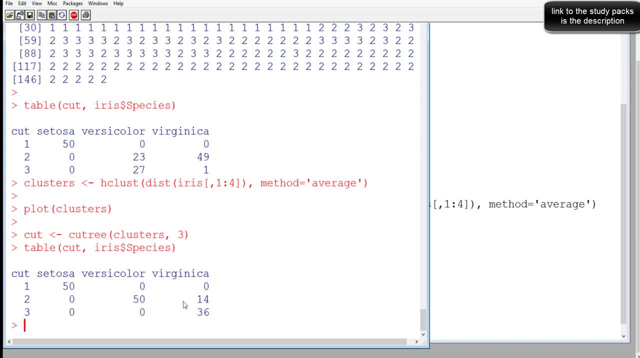 as many possible models and do the comparison in some way or the other. Thank you, 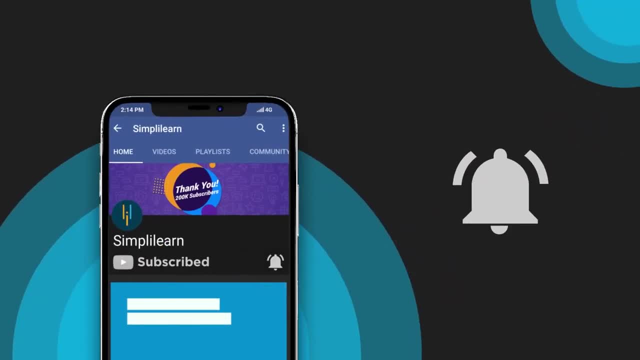 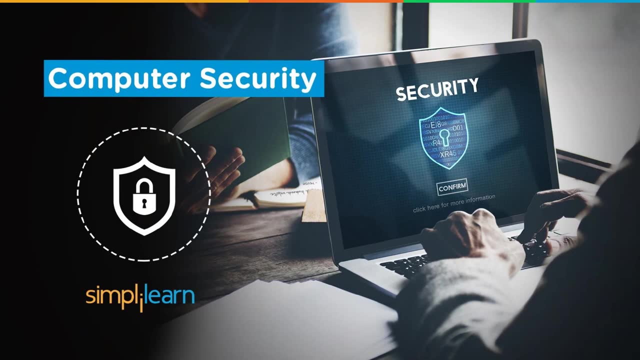 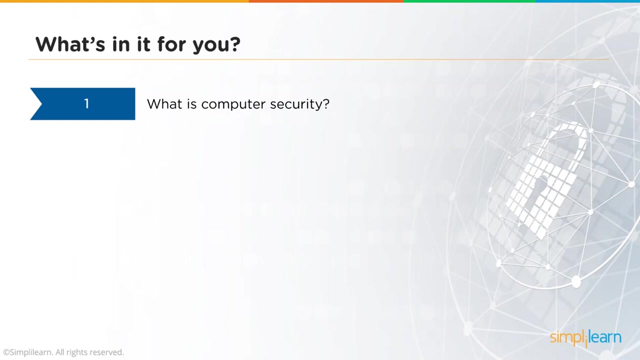 Good morning everyone, and welcome to the next video in the information security space. This video is going to deal with computer security. So what are we going to cover in this video We are going to start with. what exactly is computer security? What are the types of attacks? 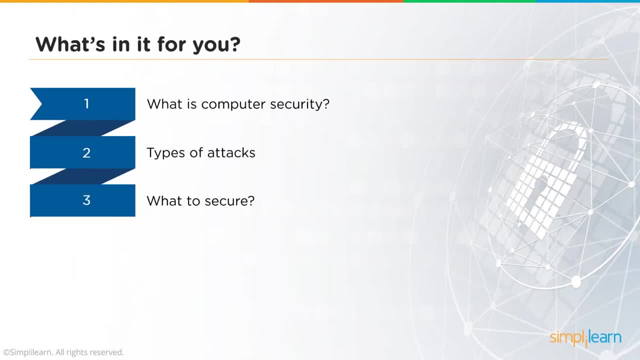 that are possible on computers. What is it that we want to secure when we say we want a computer to be secured properly? Why do we get attacked in the first place, and how to secure a computer? So let's start with the first topic. What is computer security? Computer security is the